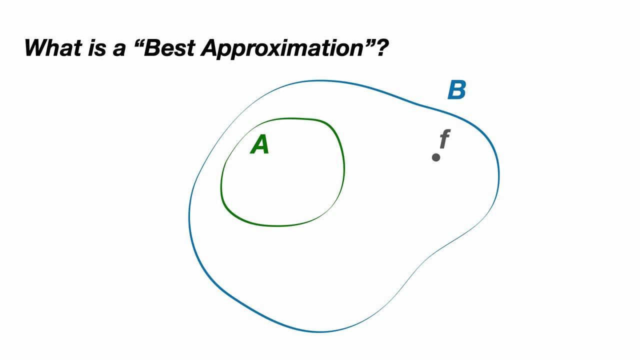 Because this is a metric space. we have a measure of the distance between any point in A and F. Therefore we say the best approximation from capital A to F is the element in capital A with the smallest distance to F, And we call this A star. 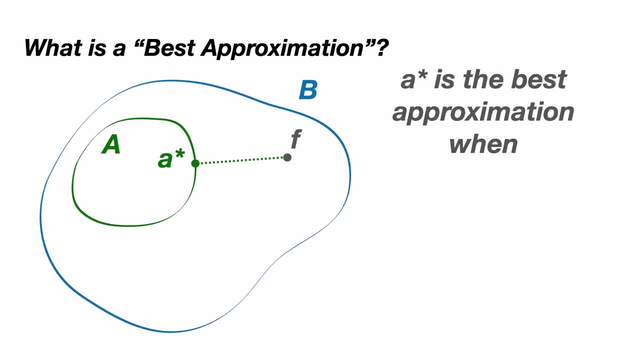 More formally we say: A star is the best approximation from capital A to F if the distance from A star to F is less than or equal to the distance between F and any other A in the set capital A. The previous definitions were a little abstract so let me give an example. 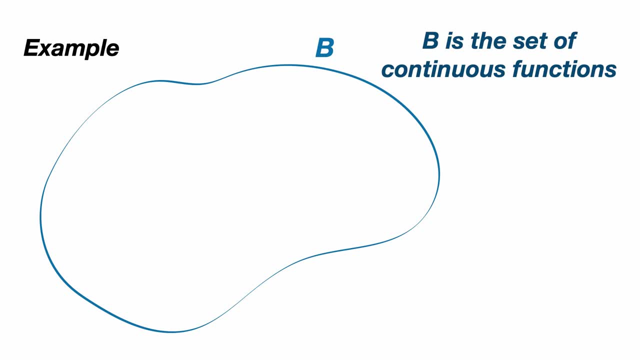 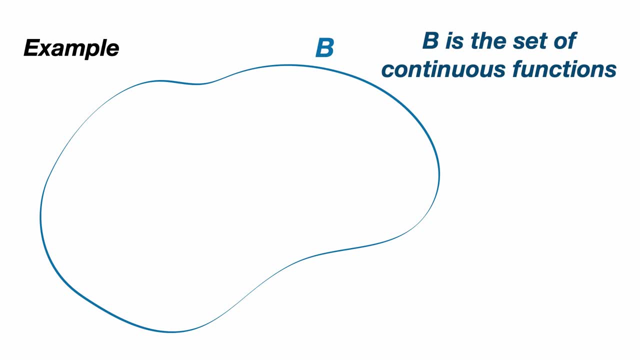 Let capital B be the set of continuous functions over a given interval. Let capital B be the set of continuous functions over a given interval and let's choose an element of capital B. Let's say f is equal to e to the minus x. 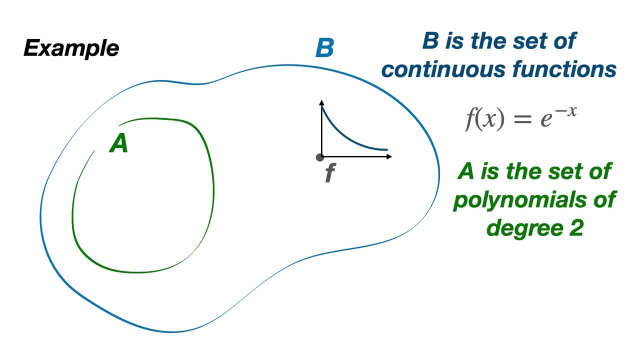 Let capital A be the set of polynomials of degree 2 and notice that this is a subset of continuous functions. We can then define the distance between any function a in capital A and f as a L2 norm of a minus f over the interval, In this case, the best approximation from capital A to f. 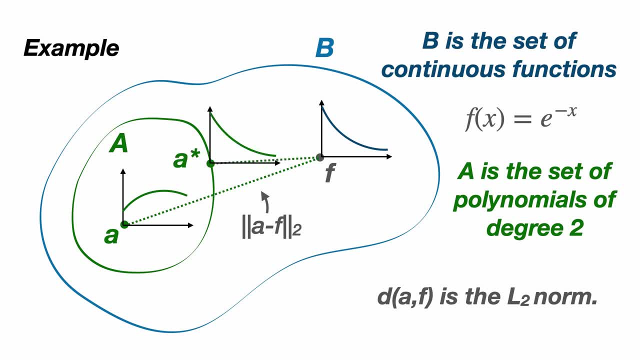 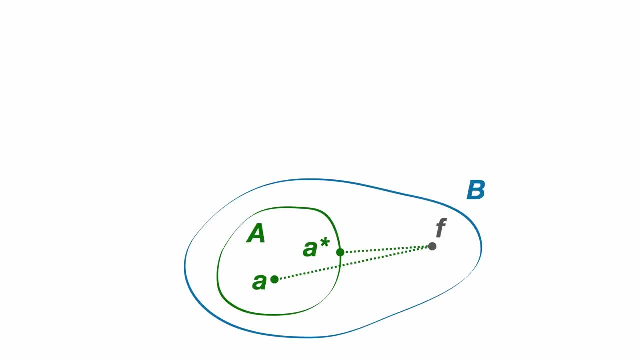 is the function a star, which minimizes the L2 norm of a minus f. We'll now show that this so-called best approximation exists regardless of which f we choose. Stated as a theorem, we say that if capital A is a compact subset of a metric space, capital B, then for every f in capital B we have 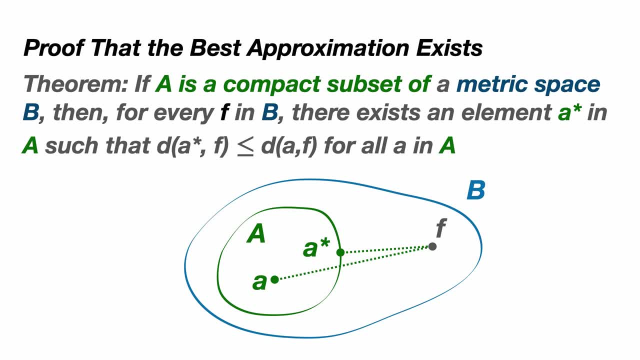 a complex subset of a metric space: capital B. If capital A is a compact subset of a metric space b, there exists an element, a star, in capital a, such that the distance between a star and f is less than or equal to the distance between f and any other element in capital a. notice that 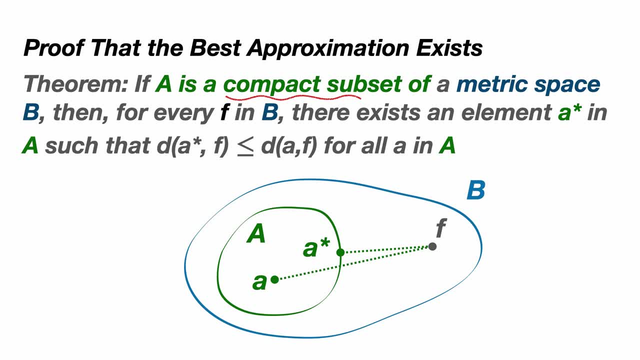 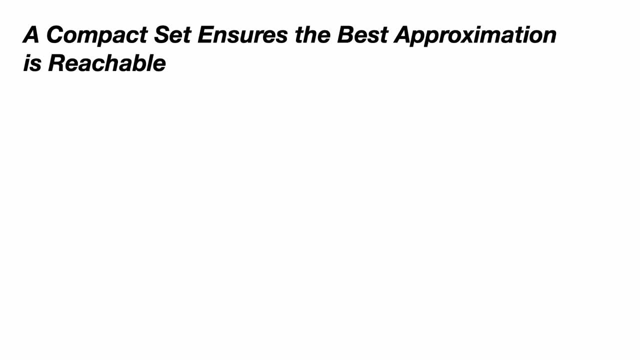 we are dealing with a compact set of approximations. let me first explain why, before getting into the proof. the compactness of our approximation set capital a ensures that the best approximation can be reached. a compact subset of a metric space is closed and bounded. consider approximating the. 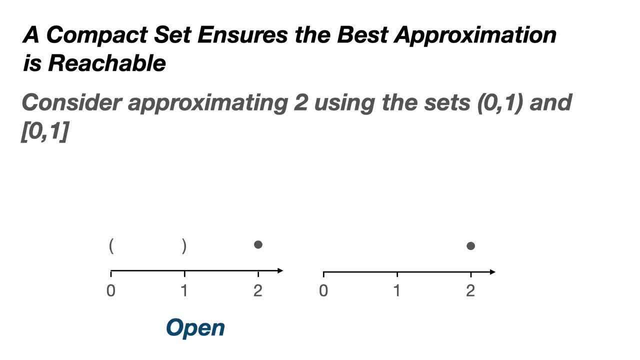 number two and you're given two sets: the open interval from zero to one, which doesn't include the end point- zero and one- and isn't compact, and the closed interval from zero to one, which does contain the endpoints and is compact. In the open case, we can create a sequence of numbers. 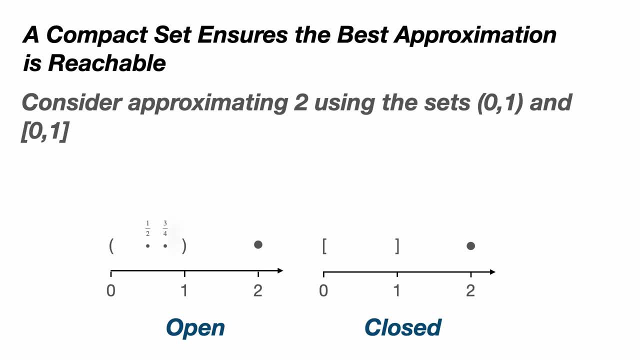 which get closer and closer to one, which of course would be the best approximation to the number two. but we never actually reach the best approximation because it isn't in the open interval. Therefore, for any approximation in the interval, you can always find a better one. In the case of the 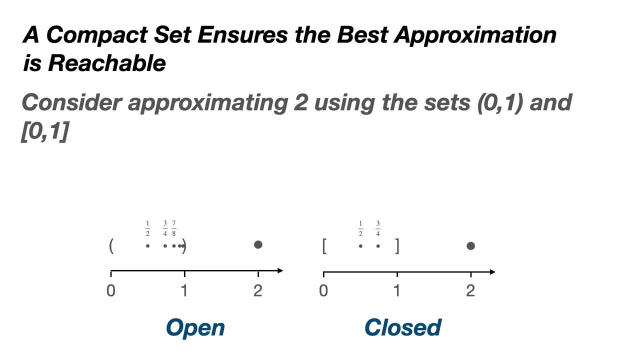 closed interval, we find that the same sequence converges to one, and one is in fact in the set. since no other number in the closed interval from zero to one is closer to two than one, we found the best approximation. So taking the distance function as a function of 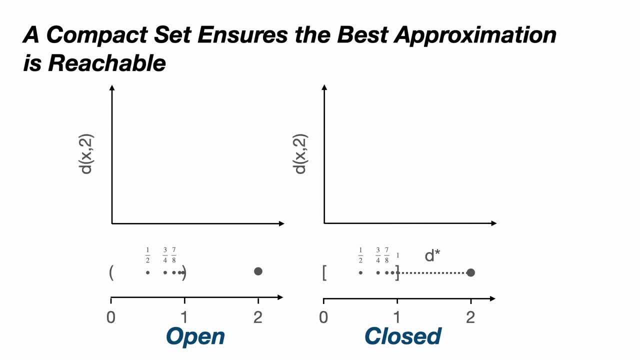 x in our open and closed intervals. if we plot the distance between x and two, we can draw a line to our map. If we plot the distance between x and two, we can draw a line to our map. minimum distance d star, which has a value of 1 and occurs when x is equal to 1 in the open case. 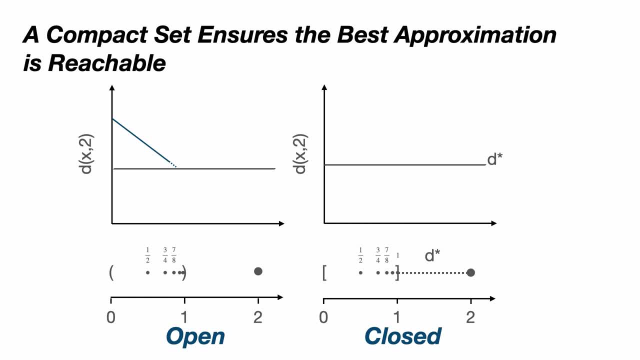 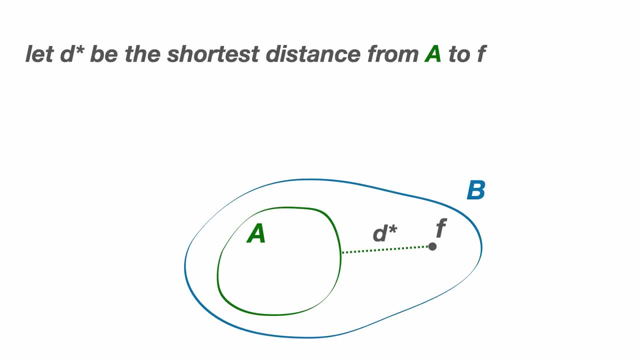 although the distance function approaches the minimum distance d star, it never actually reaches it. on the other hand, the distance function on the closed and compact set actually reaches the minimum distance d star. so we've established that there exists a minimum distance between f and the set of approximations capital, a, and we call this distance d star. we now need to show that there is. 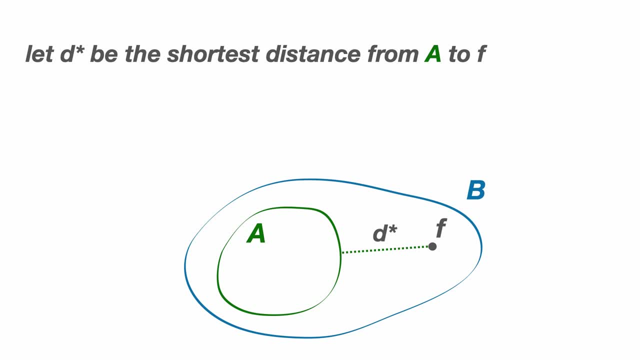 an element of this set, which actually is this distance from f and is closer to f than any other element in capital a, or at least the same distance. this is where the compactness of capital a becomes very useful. we can say that there exists a sequence of elements, a sub i, in capital a. such 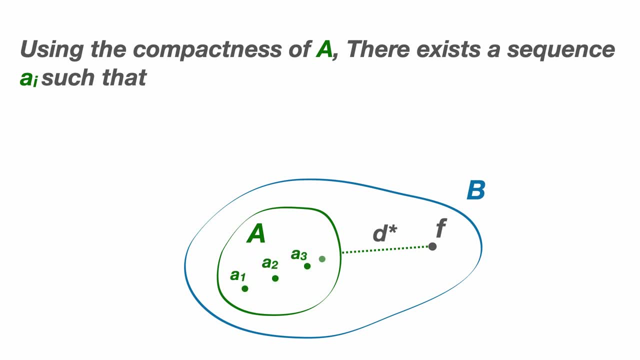 that the distance between a sub i and dx of x is equal to the minimum distance of some sum of elements in the model, which is equal to the minimum distance d square, which is equal to the minimum distance and f converges to d star. as i tends towards infinity, Let's call the limit point of this. 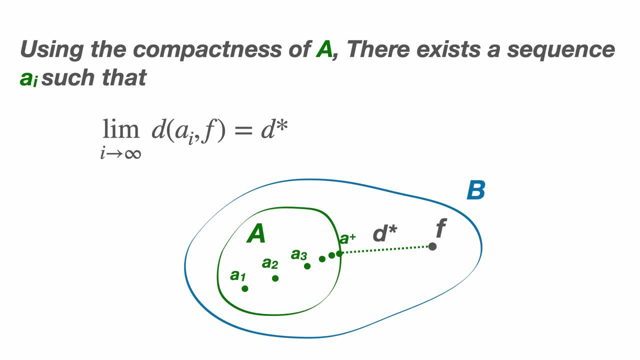 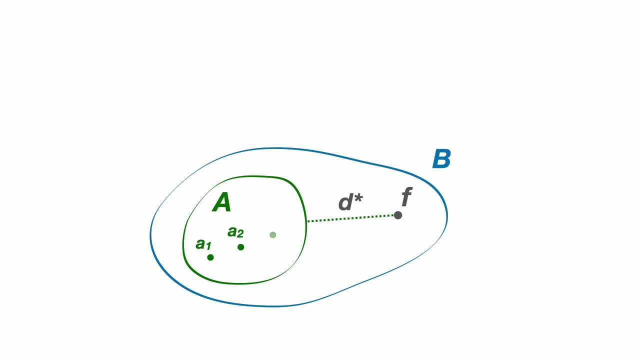 sequence a plus and to give away the ending. we'll now show that a plus is the best approximation to f. To show that a plus is the best approximation, we need to show that no other element of capital, a, is any closer to f. Consider the area immediately around a plus, Since a sub i tends to a plus, and. 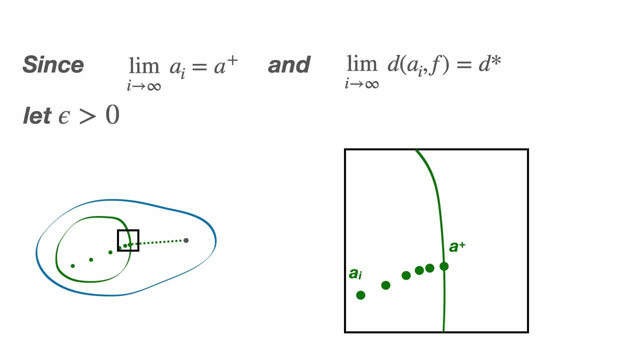 the distance between a sub i and f tends to d star. let epsilon be a small number greater than zero. If we construct an open ball around a plus with a radius of epsilon over two, we can guarantee that there will be some number greater than zero. 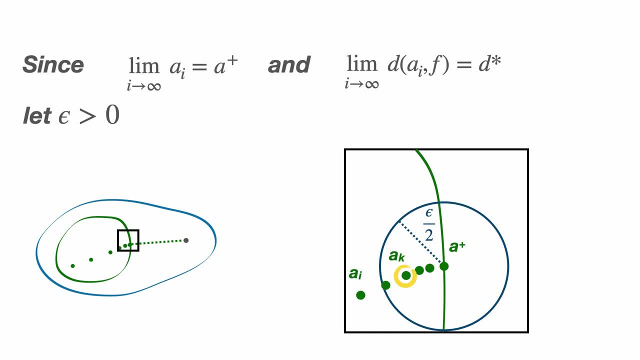 k, such that a sub k lies within this ball. This implies that there exists an element, a sub k, which simultaneously has a distance less than epsilon over two away from a plus and a distance less than d star plus epsilon over two away from f From the triangle inequality. we have the. 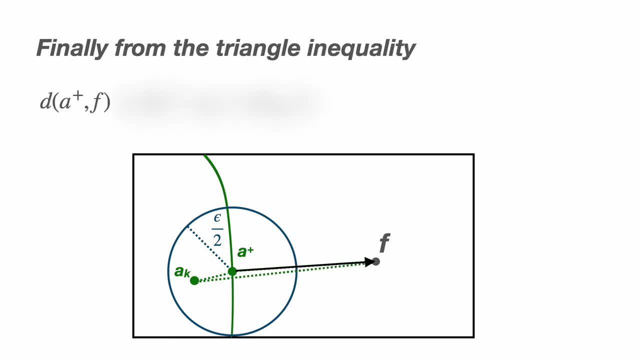 distance between a plus and f is less than or equal to the distance between a plus and a sub k plus the distance between a sub k and f. Now we already have inequalities for both of these distances on the right hand side, and adding these together shows that the distance between a. 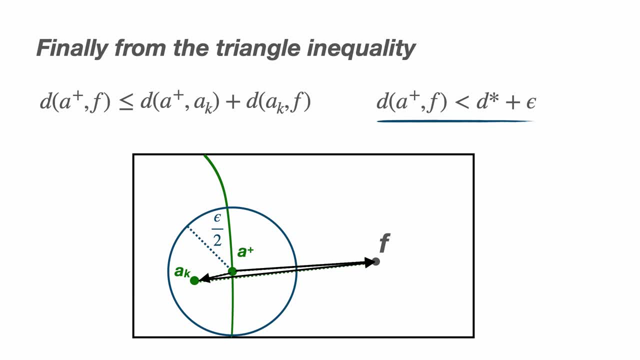 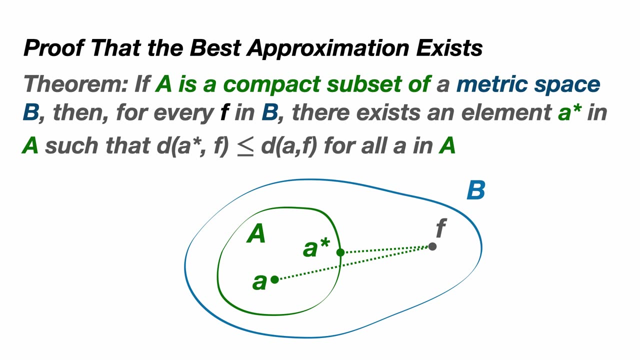 plus and f is bounded by d star plus epsilon. Since epsilon can be made as small as we choose, then the distance between a plus and f is d star, and so a plus is the best approximation. So there we are. we've found that when making approximations in a metric space, it's possible to show that there's at least one point, a star, in capital a, our set of approximations, such that no other a in capital a is closer to f, and a star is therefore the best approximation from capital a to f.